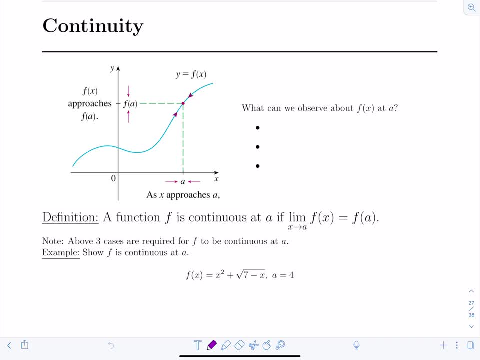 This is Calculus 1, video lecture number 5 on continuity. So to begin our discussion, we're going to look at this graph here of some function: y equals f of x and we want to observe the behavior of this function at a where x is equal to a right here. Okay, so what can we observe? 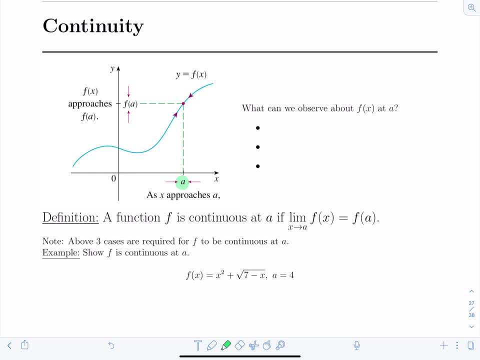 about f of x at a. Well, one thing we notice is that our function is defined at a meaning. if I plug in a for x, the function has a value f of a. So we can say that f of x is defined at a. All right, what else can we say? Well, we've been talking a lot about limits lately, so 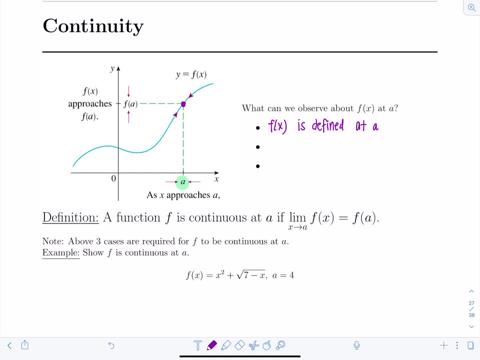 let's say that f of x is defined at a. Let's see as x approaches a from either the left hand side or the right hand side. what is f of x doing? Well, from the left hand side, the graph f of x is approaching f of a. and also from the right. 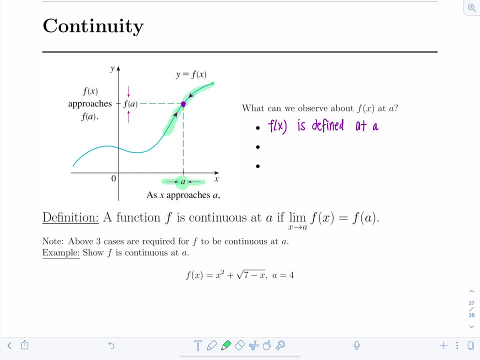 hand side. as x approaches a, the function is approaching that same value. So we can say that the limit exists. It's clear that the limit from the left of a of the function equals the limit from the right of a, So we're going to write that the limit as x approaches a of f of x exists. 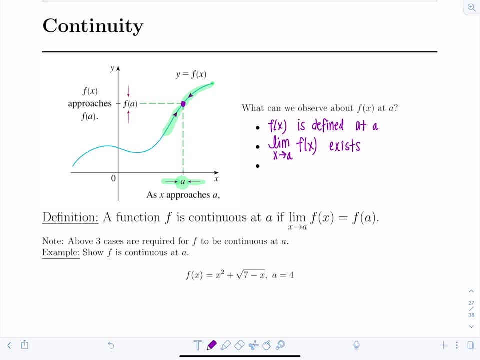 And the third thing that we observe is that the function value f of a is equal to the limit. So the limit as x approaches a of f of x is equal to f of a, And this is our three-part definition for continuity. So the definition is as follows: 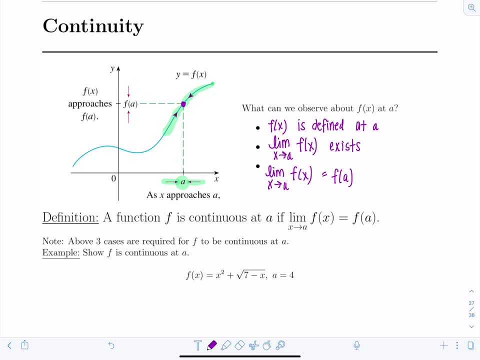 If f of x approaches a of f of x is equal to f of a, The function f is continuous at a if the limit as x approaches a of f of x equals f of a. So there's three conditions that need to be satisfied in order for a function to be continuous. 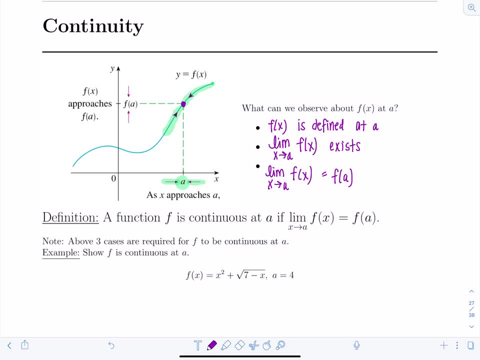 at a point. The first is that the function has to be defined at that point. The second is that the limit as x approaches a of f, of x, has to exist as a finite number. And then the third is that the function value has to equal the limit. But if you just write that third statement, that the function 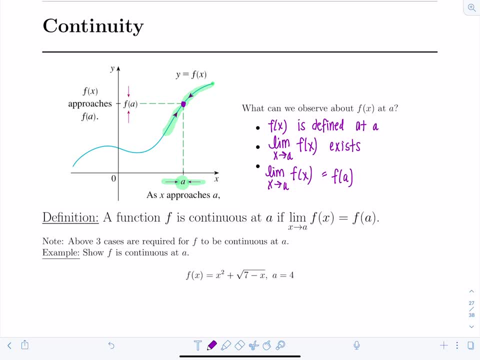 value equals the limit, then that automatically guarantees that the first two are satisfied, Because if the function's not defined or if the limit doesn't exist, then obviously the third condition is going to fail. Okay, so let's look at how we can prove or show that a function is. 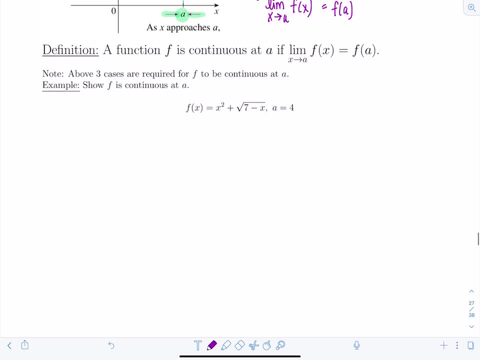 continuous at a certain point, a, using this definition. So show the following function: f of x is continuous at a, And here we have f of x defined to be: f of x is continuous at a x squared plus radical 7 minus x. And the point that we're interested in investigating is where. 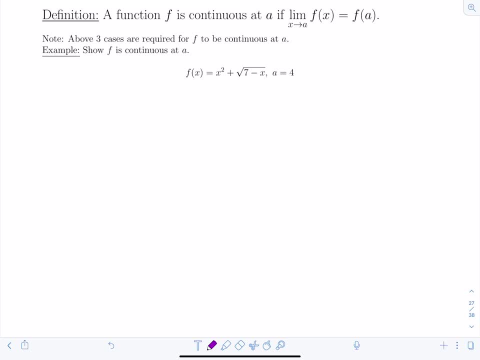 a equals 4.. Okay, a is the x value. So the first condition that needs to be satisfied is that I have to show f of x is defined at a equals 4.. All right, well, how do I know whether or not the function is continuous at a? 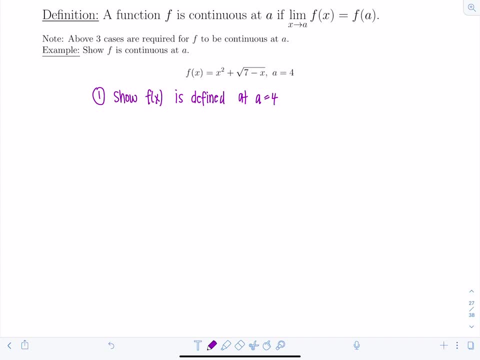 Well, I need to figure out what the domain of this function is and see if 4 lies within that domain. So can we identify what kind of function we're working with. Well, this function, it's a combo, right, It's a radical function. And that x squared term, that's a polynomial And it's a. 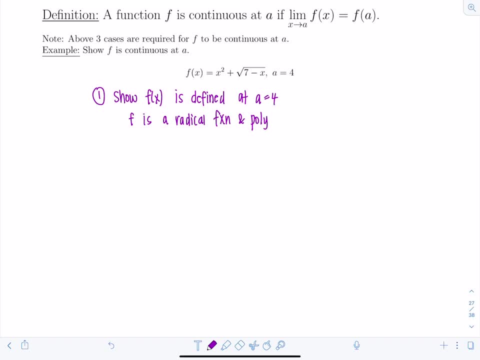 polynomial, So it's a combo. The domain is going to be restricted because of that radical right. The index is even Polynomials. we know their domain's, all real numbers, But we have the condition that 7 minus x has to be greater than or equal to 0, because we can't take the square root of a negative quantity. 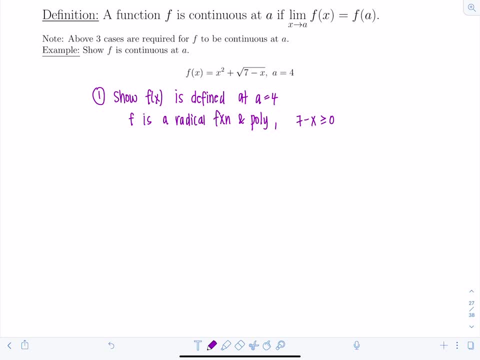 So if I solve this inequality, that's going to give me the domain for this function, namely that x is less than or equal to 7.. So the domain for f of x is from negative infinity to 7.. And notice, we're studying or investigating the continuity at a equals 4.. 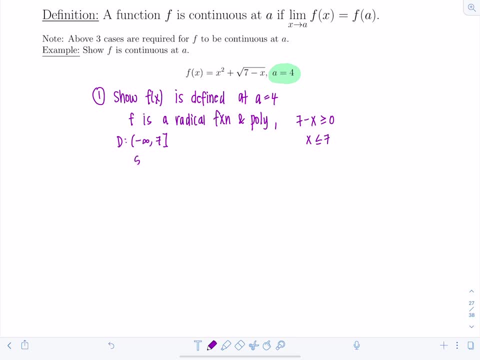 Well, 4 belongs to the domain, right? And you can write that, since 4 is an element of or belongs to the domain, using this notation, that means it belongs to the domain. Then we can say that f of x is defined at a equals 4.. So that's good to go. First condition satisfied. Second condition: 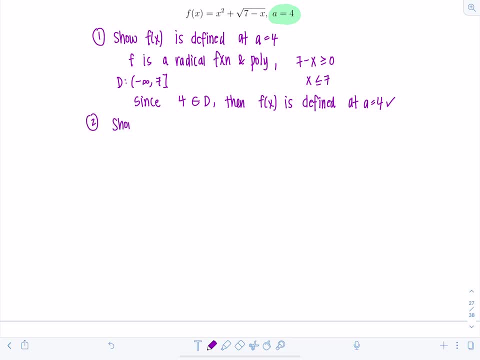 I need to see if the limit as x approaches a, in this case 4 of f of x, exists. Can we take this limit? Well, let's see. I have the limit as x approaches 4 of x squared plus radical: 7 minus x. 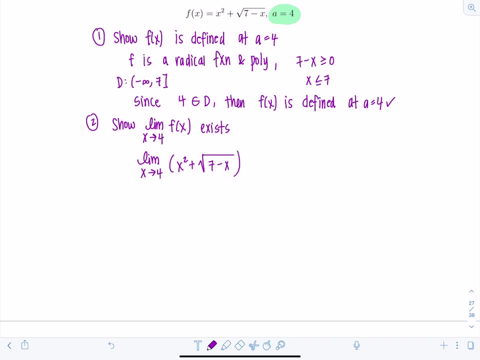 How do I take this limit? Well, we use direct substitution right as our first kind of go-to, And then, if we run into problems, we do something else. But let's see, can we directly substitute? Sure, no problem, Why not? So this is going to be 4 squared plus. 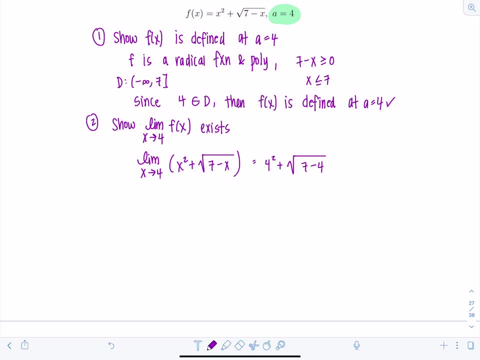 radical 7 minus 4, which is 16 plus rad 3.. Okay, looks good. Now let's see here the third condition. I have to see if step 1, equals step 2.. So basically, I want to show that f of 4 is equal to the limit. 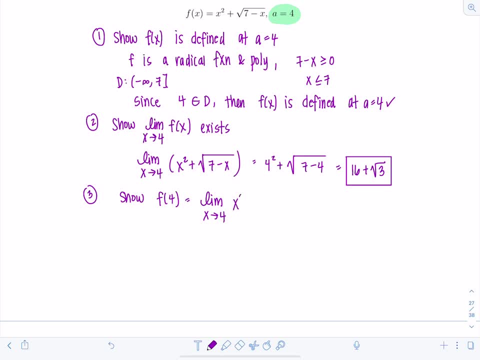 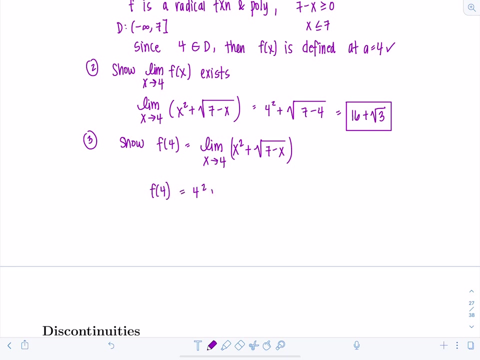 as x approaches, 4 of x squared plus rad 7 minus x. Is that true? Well, how would you figure out what f of 4 is? You would just directly substitute it in as well. So 4 squared plus rad 7 minus 4. 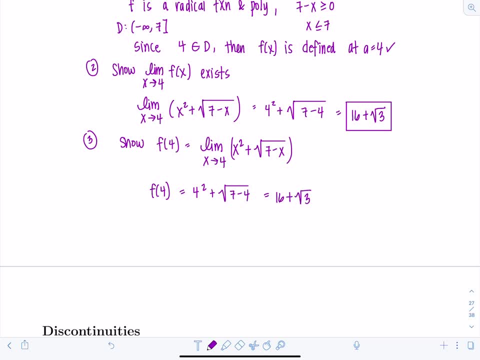 that's 16 plus rad 3.. So yeah, that checks out. Okay. so there, we've tested all three conditions at a specific point for continuity. Now, what does it mean when a graph is not continuous? Well, there's varying kinds of discontinuities. 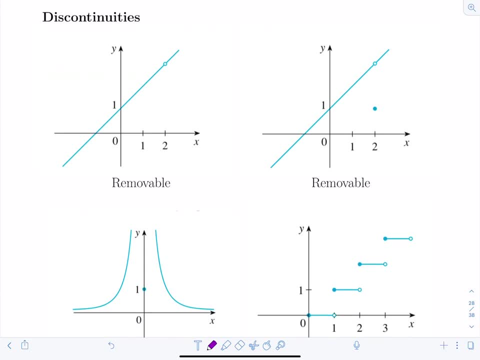